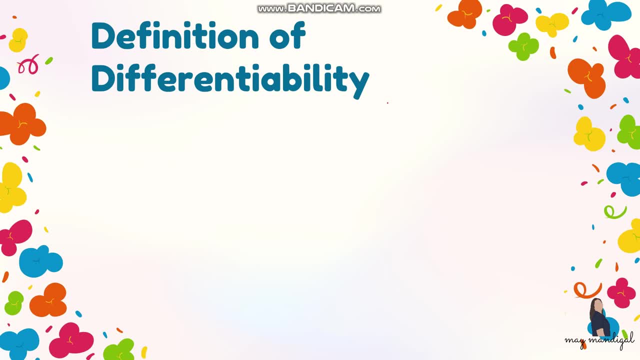 how about differentiability? So what's the definition of differentiability? So we say a function is differentiable at x equals c if the derivative f prime of c exists. So a function is differentiable at a certain point if f prime of c exists. Okay, now how are we going to check if f prime of c exists, given that x is? 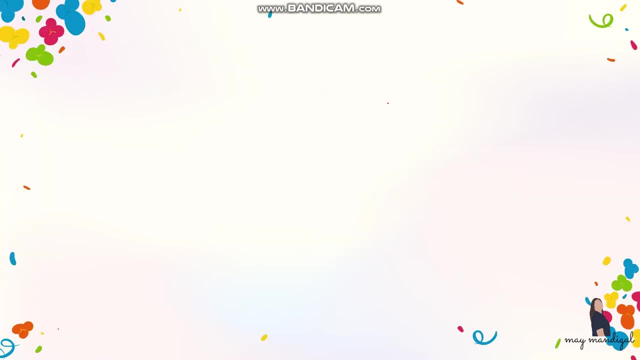 equal to c. So we have to solve for the right hand derivative and the left hand derivative. So what is the right hand derivative? So let y be equal to f of x. It's b, defined at x, equals c. So the right hand derivative is the derivative of f, prime of c. So we have to solve for the. 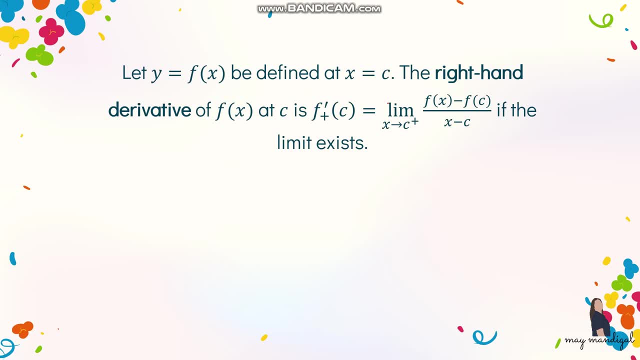 right hand derivative of f of x at c is defined by this formula. So we have to use the limit, So limit of f of x minus f of c, all over x minus c, as x approaches c from the right. So that is how we are going to identify our right hand derivative, So f of x. so that is our function. 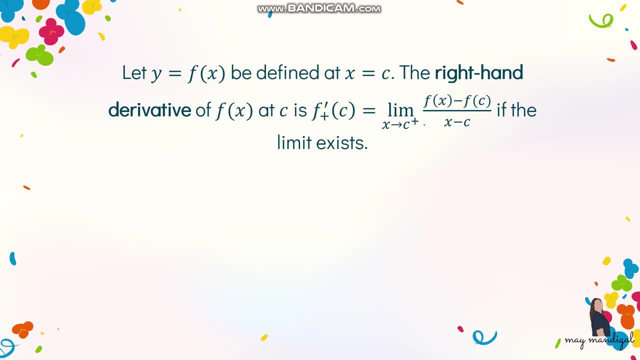 then f of c, so you just have to substitute the given c to the function and whatever value we will get. So f of x is the right hand derivative of f of x at c. So that is how we are going to identify our right hand derivative of f of x at c. So that is how we are going to identify our. 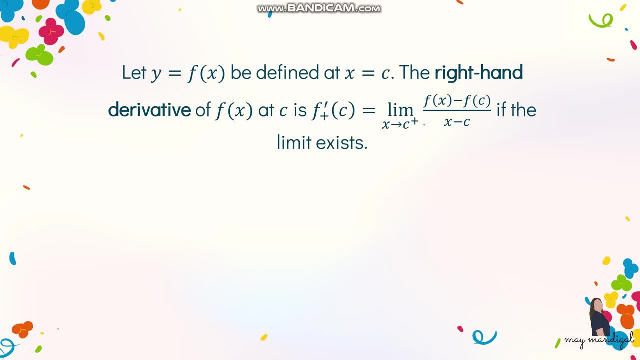 That's the one that they will put there All over x minus c. So that is our right hand derivative And we also have to solve for the left hand derivative. So we will be using the same formula but we get the limit of that function as x approaches c from the left. 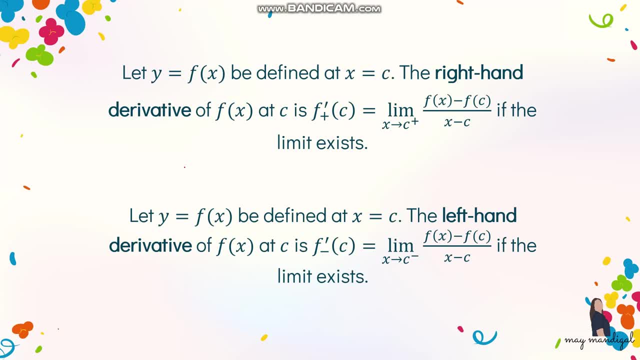 Okay, so that will be our left hand derivative. Now, when can we say that our f prime of c exists? So f' of c exists at a given value of c if the right-hand derivative is equal with our left-hand derivative. So we have to check first if these two values are equal. 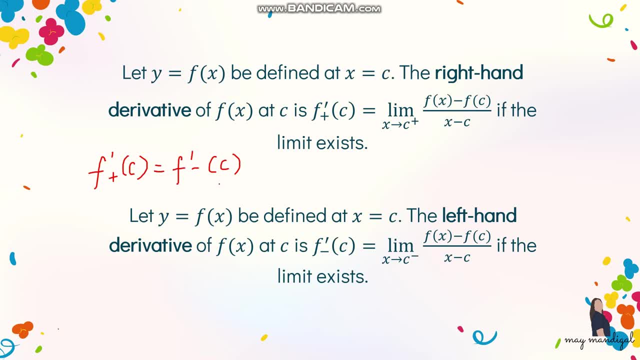 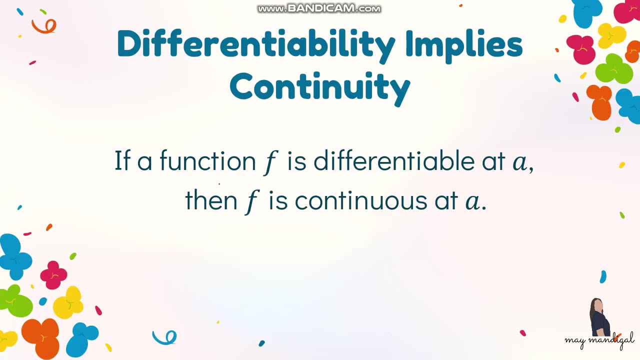 Then, if they are equal, we can now say that our function is differentiable because it means that f' of c at a given value of c exists. Now, what's the connection between differentiability and continuity? So differentiability implies continuity. 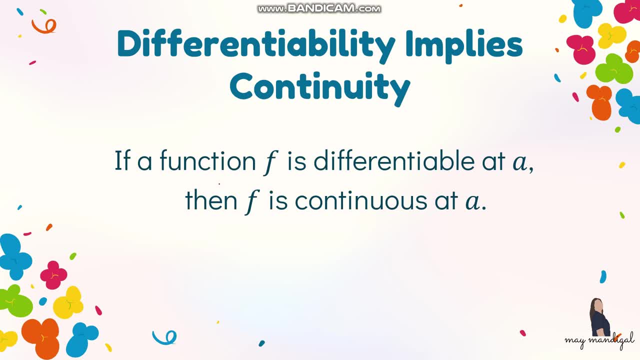 So what does it mean? If a function f is differentiable at a, then f is already continuous at a. So once we already prove that a given function is differentiable at a certain point, then we can also say that that particular function is also continuous at that given point. 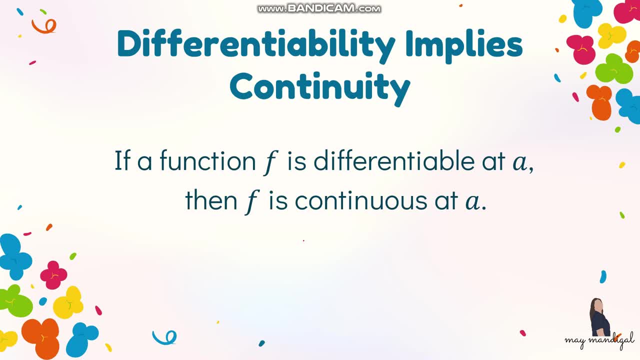 So another thing that we can get here is, if the function is not differentiable at a, then that function is not continuous as well at that particular value, a. But continuity does not imply differentiability. Okay, So that's one thing that we have to remember. 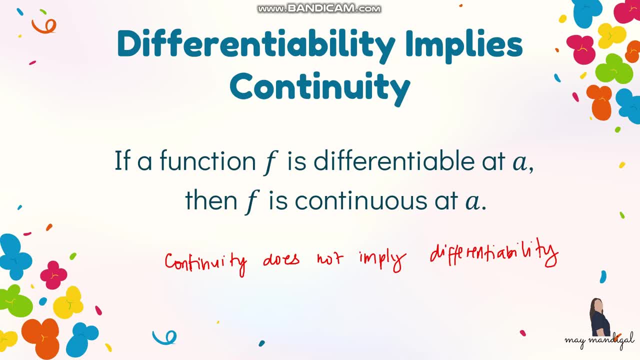 Continuity does not imply differentiability, because a function can be continuous at a given point, but it may not be differentiable at that particular point. Example. So I will be showing you examples of graphs. So let's say this graph number one here: 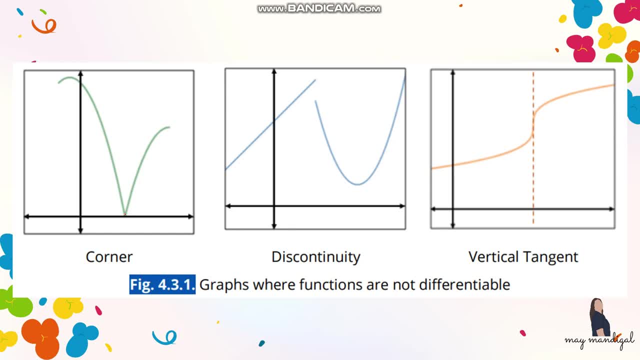 If your function has a corner like this one. So this function is continuous, as you can see, but at this certain point, this one right here, our function is not differentiable, because if you will be getting the right-hand limit and the because, if you will be getting the right-hand derivative and the left-hand derivative, the two will be different in value. 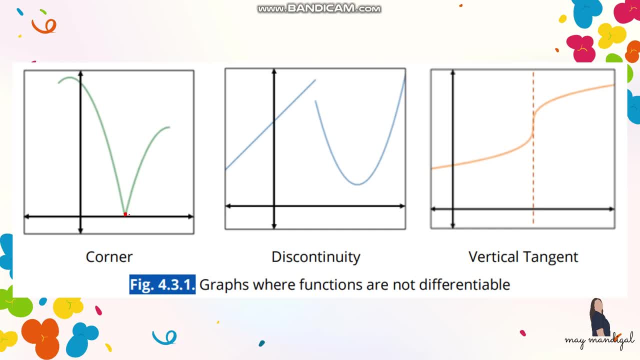 Okay, So if there's a corner in our graph, So automatic, that is not differentiable. Okay, So this is one example wherein a function is continuous but not differentiable. However, if it's discontinuous, like this second graph, 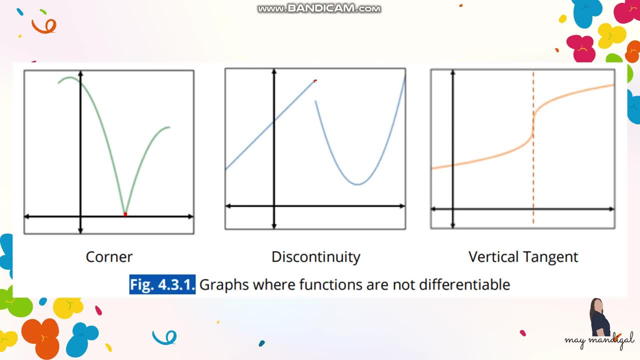 So, as you can see, there is a gap between our graphs here. So these two points right here. So if you will see, this is it shows discontinuity. So if it shows discontinuity automatic, It is not differentiable as well. 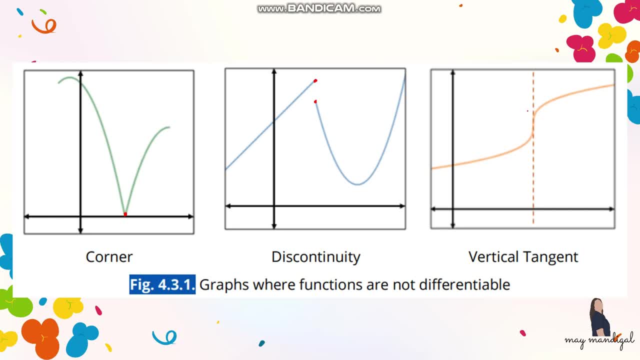 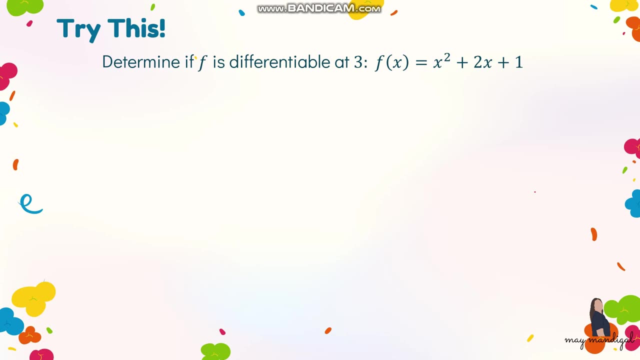 Okay, and then here, this one is an example of a graph that is continuous, But again, it's not differentiable, because- and we have here a tangent, a vertical tangent. Now let's try to determine if the following functions that I will show you are differentiable at specific points. 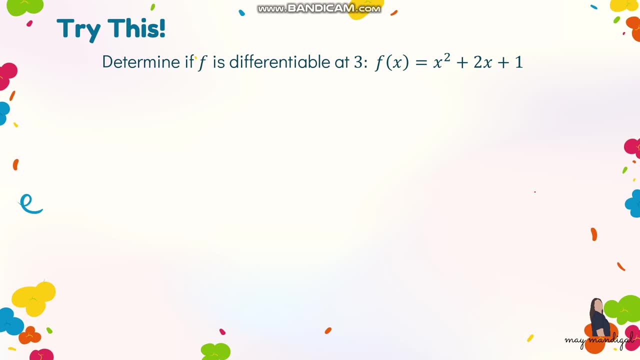 So first determine if f is differentiable at 3. So we have f of x equals x squared plus 2x plus 1, but since this is quadratic function, we can say that it is continuous. okay, but again, we cannot assume that if it's continuous. 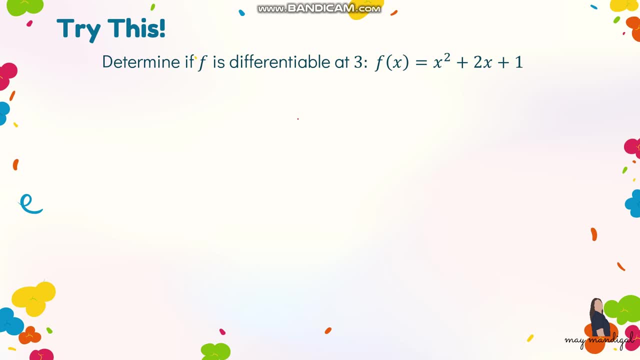 automatic. it's differentiable, so we have to check. so what we will do is we have to get the right-hand derivative and the left-hand derivative, so right-hand derivative and the left-hand derivative now in our formula, so we have their limit of f of X minus f of C, all over X minus C. so before you start, let's try to. 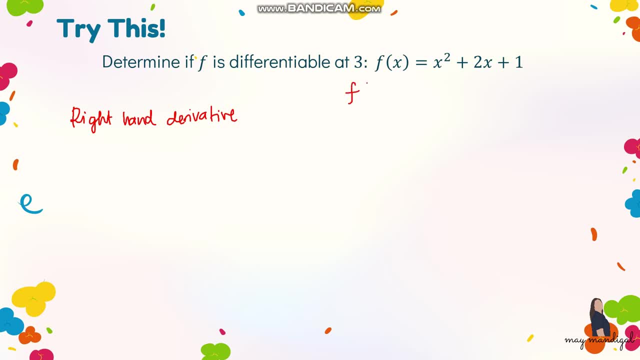 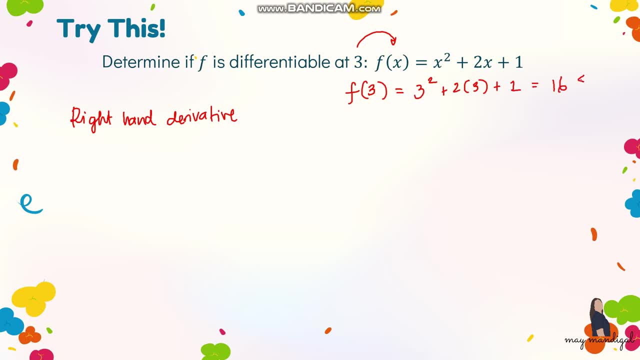 to 16. so this is our f of C. okay, so here that's all for the right-hand derivative. so we know that the right-hand derivative at x equals C of our function is just equal to getting the limit of F of X minus f of C all. 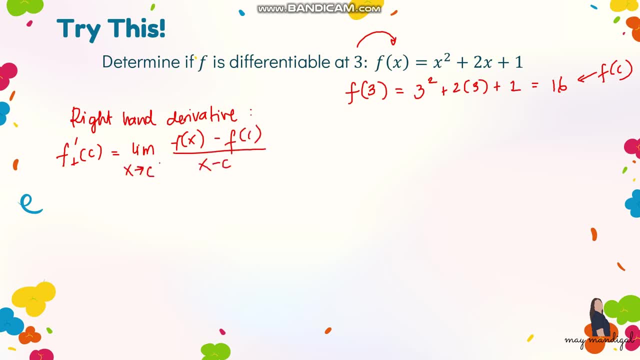 over X minus C as x approaches C from the right. so I just have to substitute everything so we have limit L: zero, zero, zero, zero, zero, zero, one, zero, zero, zero it. our c is 3, so 3 from the right, f of x is you just have to copy the function so you have x. 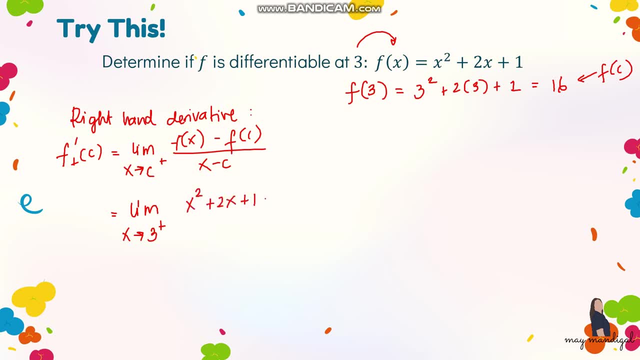 squared plus 2x plus 1 minus our f of c. so our f of c is this: 16 over x minus c, which is 3, and then all you have to do is to simplify this. so we have x squared plus 2x minus 15, all over x minus. 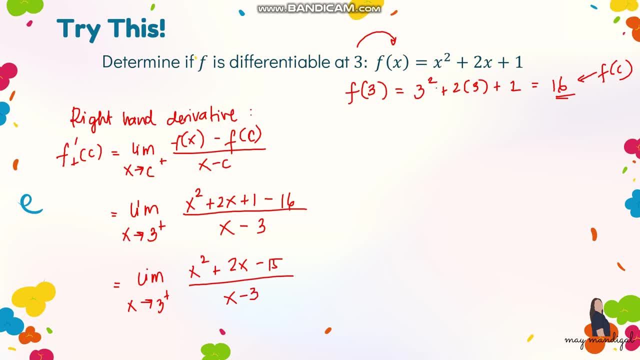 3. now, before you get the limit, we can still simplify this so we have limit. as x approaches 3 from the right, we can factor out our numerator so it will be x minus 3, x plus 5, all over x minus 3, and then we can cancel this so we will be left with the limit of x plus 5. 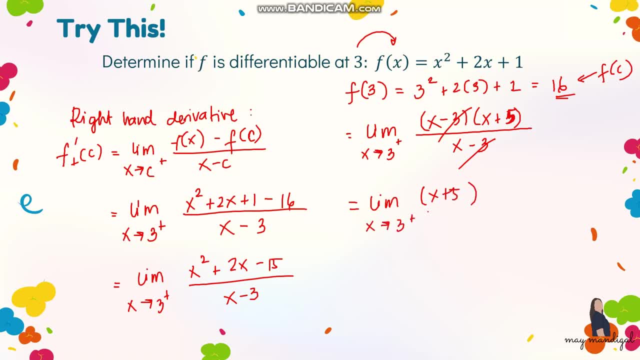 as x approaches 3 from the right. now. from here, you can now get the limit of x plus 5 as x approaches 3 from the right. since this is just a linear function, you can just substitute, so it will become a 3 plus 5. 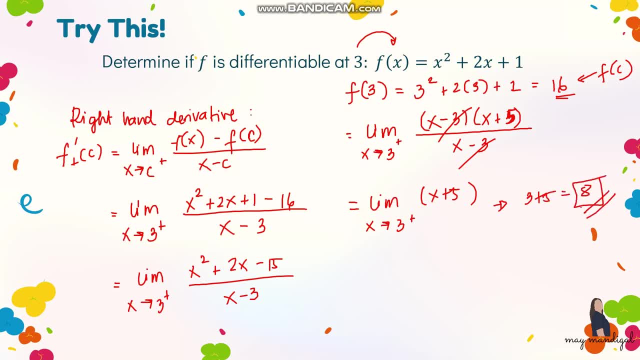 or 8. so this is now our right hand derivative. now let's get our left hand derivative. so in getting the left hand derivative, since we have the same function, there's only one function here, so we will be using that one. that will be our f of x as well. this will be our f of c, or we will. 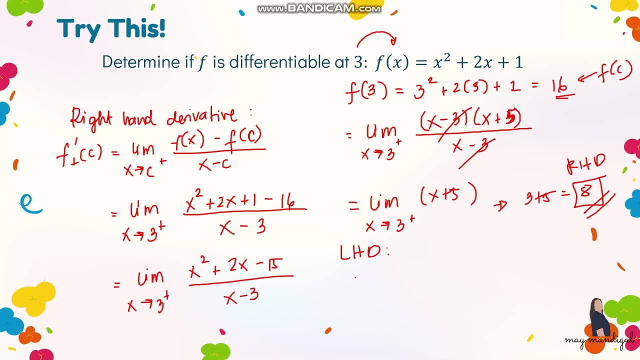 just get the same value here, which is a limit of x plus 5, and we will get the same value here. so there are 2 marginals and 2 regardingあります, and the left hand will be acting in this term. but first, first, if you have 8, 1 equal to 8.. 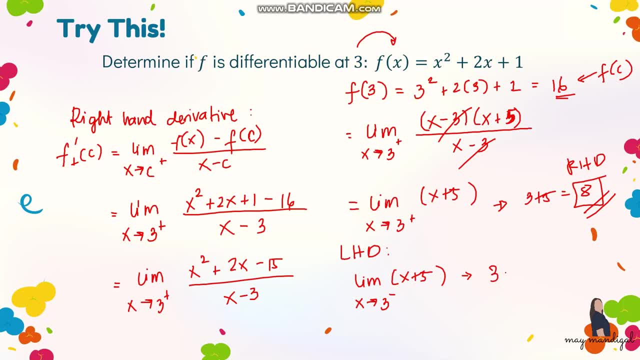 plus 5 as x approaches, then this 1, 3 from the left. so it will be like this, so you can again substitute. so you have 3 plus 5 for 8. so this is our left hand derivative now, since our right hand derivative is equal. 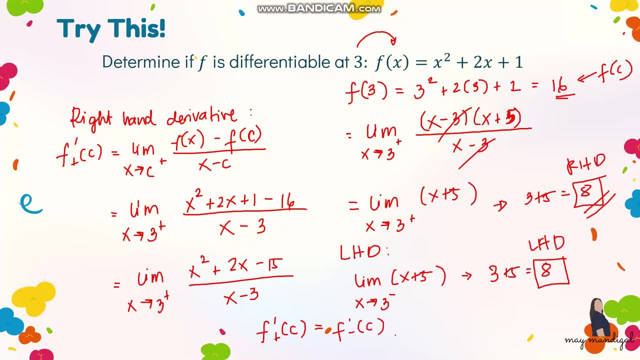 right hand derivative is equal with our left hand derivative, then we can say that ourwigth Fliness f of x, f of X is a differentiable at 3. so there, so as long as the right hand limit, the right hand derivative and the left hand derivative are equal, then 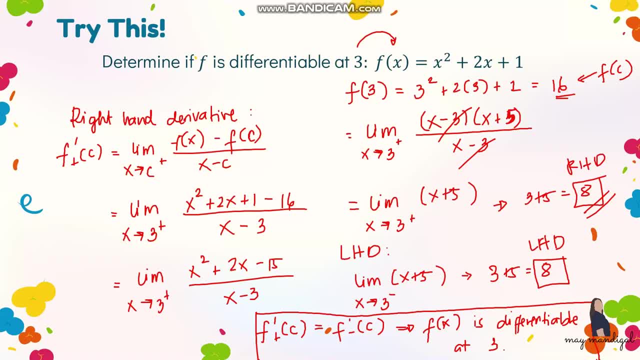 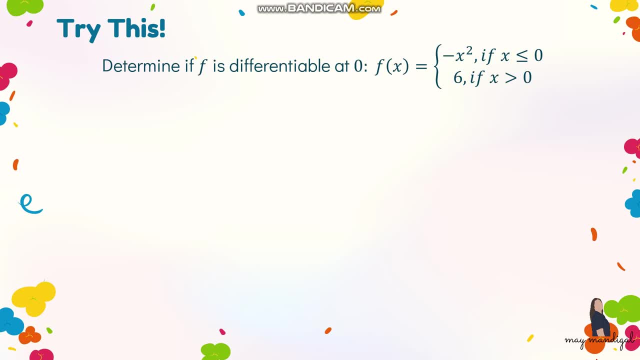 we can say that our function is differentiable at a certain point. now let's have a piecewise function here. so let's determine if the function f of X is differentiable at 0. so as you can see, we have two sub functions. we have negative X if X is less than or equal to 0. we have 6 if X is greater than 0. so 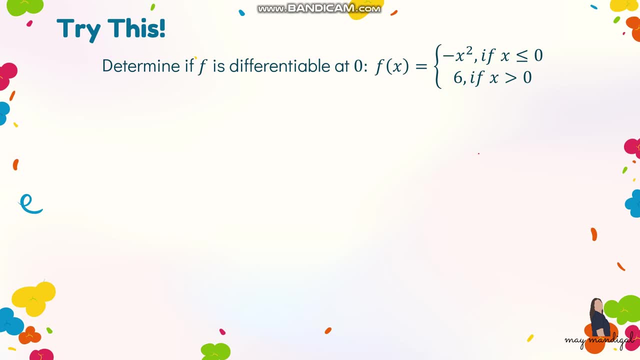 first thing that we have to do is to solve for f of C first, so that when we do our solution later on we can just plug in the value of f of C. so f of C, f of 0, this is our C now, since X is 0. so 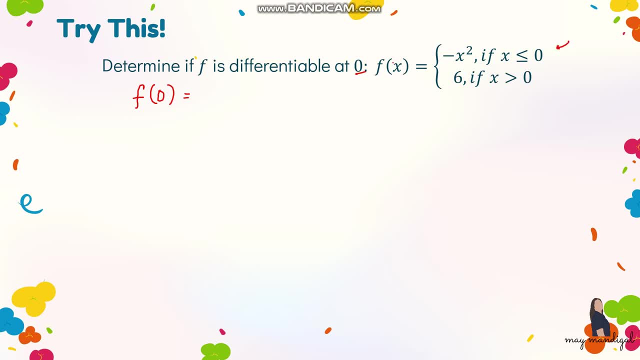 we'll be using this one, the first sub function, and then substitute here. so that's negative, zero squared or just equal to zero. so this is our f of c. now let's solve for the right hand derivative and the left hand derivative. okay, now for the right hand derivative. we know we have to get the limit of. 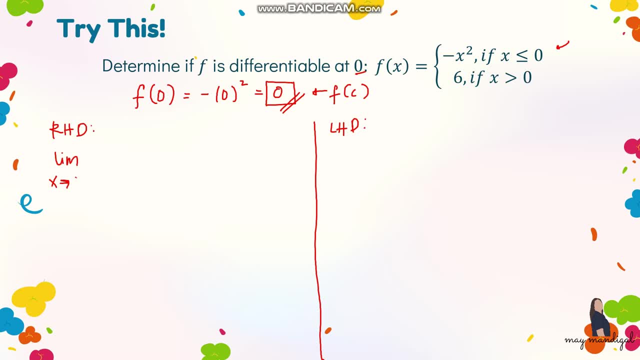 our function as x approaches c, which is zero from the right. okay, now what f of x should we use for this function, since what we want is zero from the right? so you have to get the function wherein it's greater than zero, because, again, we want to get the derivative from the right. 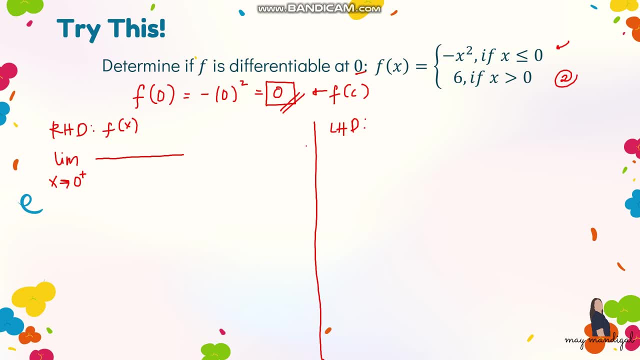 so we will be using the second sub function, that will be our f of x, which is six. okay, so you substitute, so we have f of x, so six minus f of c, which is zero, all over x minus c, which is zero as well. so if you solve this, six over x, so we have limit of six over x. 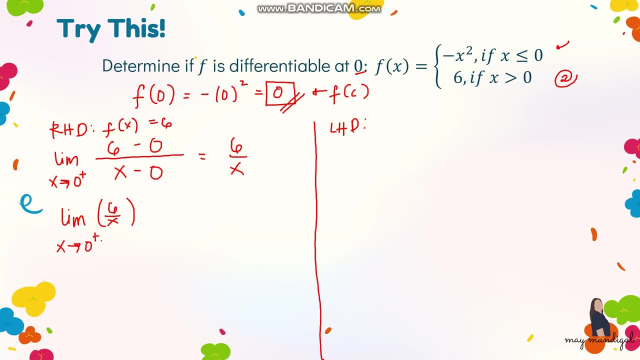 as x approaches zero from the right. so you can just substitute. but if you substitute that we will get six over zero. or if it is undefined, that means the limit does not exist. so that means, since the limit does not exist, therefore we don't have the right hand derivative. 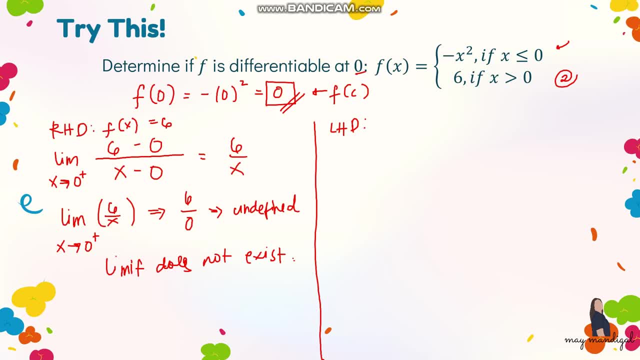 so actually you can stop here, but let's just try to solve for the left hand derivative using the limits. so limit as x approaches zero from the left. this time our f of x will be the sub function wherein x is less than zero, which is the first one. so that will be our f of x. 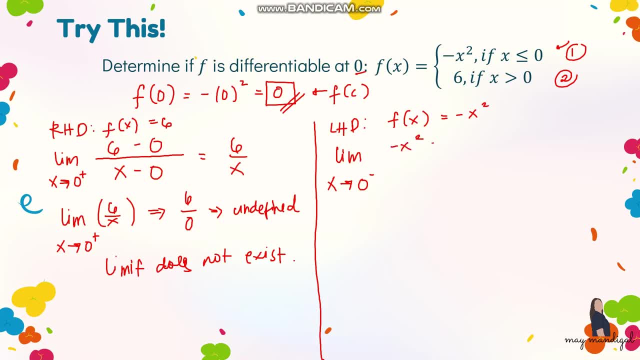 so you have negative x squared minus and then our f of c, which is zero, all over x minus zero. you can just simplify this: negative x squared over x, or what we will have here is negative x as x approaches zero from the left. so you can just substitute, or the limit will be zero. 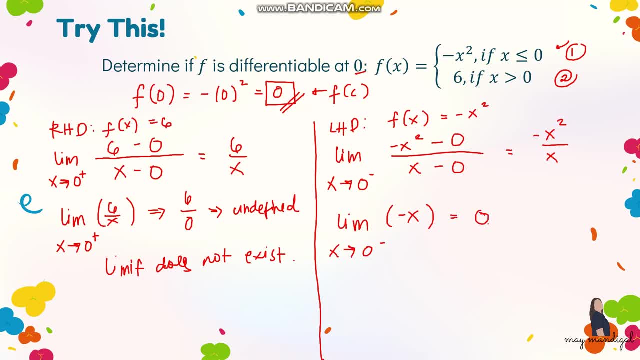 okay now, since the limit is zero for the left hand derivative, so there is a value here. but since our right hand derivative is zero, so we will have negative x squared over x, minus x squared over x. so if the left hand derivative at x equals c is not the same as the left hand derivative at x equals c. 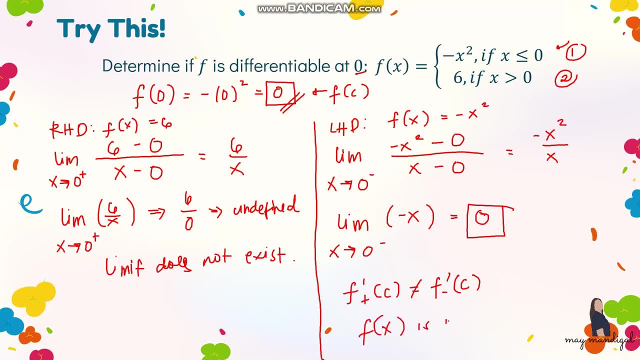 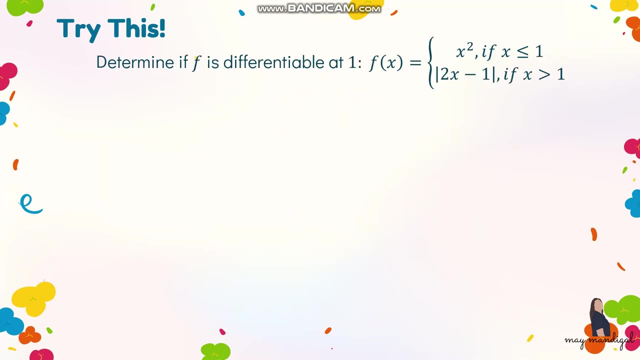 then f of x is not differentiable at, x equals zero. so that will be our final answer. another example: determine if f is differentiable at one. so we have f of x equals. we have a piecewise function, again x squared. if x is less than or equal to one, we have the absolute value of 2x minus one. 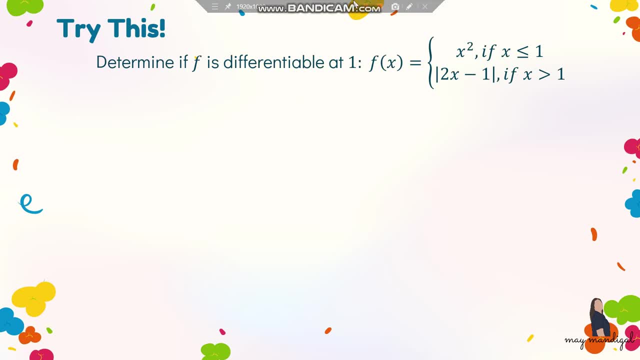 if x is greater than one. so first let's solve for f of c, so that we can just plug in directly our value. so c is one. so since c is one, we will be using the first sub function in solving our f of c. so that will be. 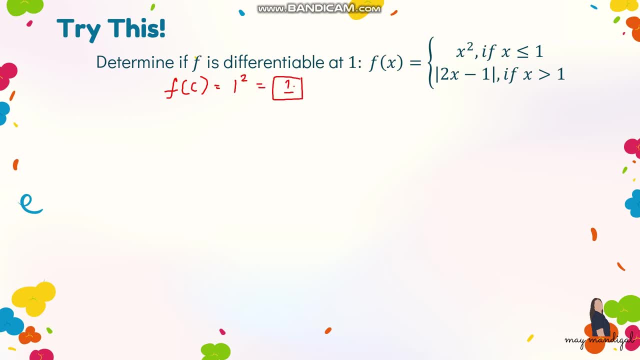 one squared or one. so that is our f of c. so let's solve for the right hand derivative and also our left-hand derivative. so you get the limit as X approaches C, which is 1 from the right. now what will be our f of X for the right-hand derivative, since? 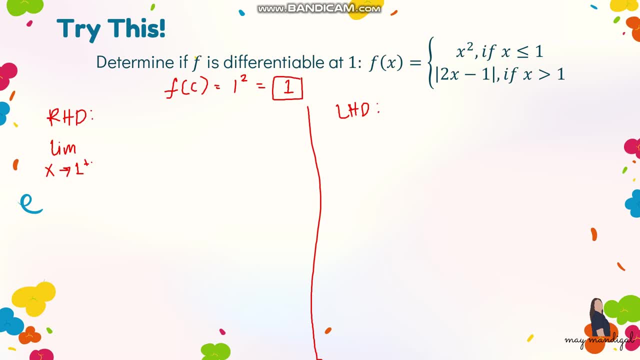 again, it's the right-hand derivative. we want to get the function sub function where in the value of X to be used is greater than 1, and that is the second sub function. so that is what they will use here. that will be our f of X here. so 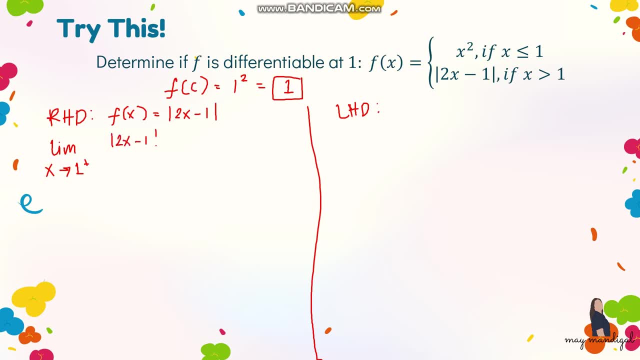 let's put here absolute value of 2x minus 1 minus f of C, which is 1 all over X minus C. so the absolute value, you can just simply remove that 1, so 2x minus 1 minus 1 all over x minus 1. simplify this so you have 2x minus 2 over x minus 1. so from here you can still. 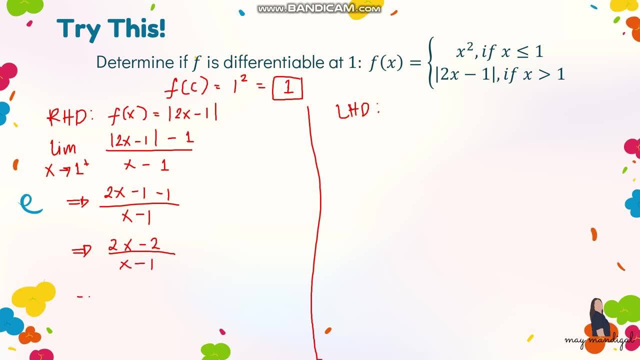 simplify this: you can factor out 2, and then you have x minus 1 all over, x minus 1, so that we can cancel this one out. therefore, what we have now is a limit of 2 as x approaches 1 from the right, and then you get the limit. since this is a constant function, the limit is just itself, which? 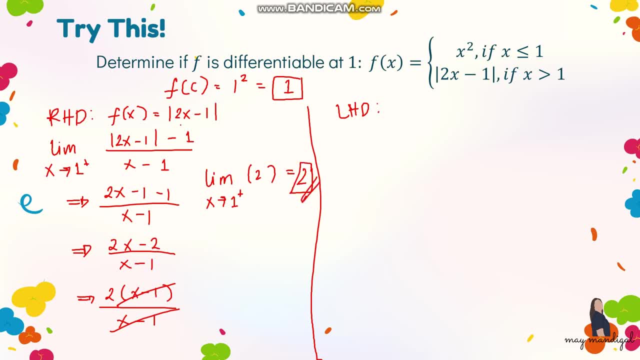 is 2. so this is our right hand derivative. now let's check if the left hand derivative will be the same. so here the f of x that we're going to use, or the sub function that we're going to use, will be x squared because it's the left hand. so that means we want to get the sub function wherein. 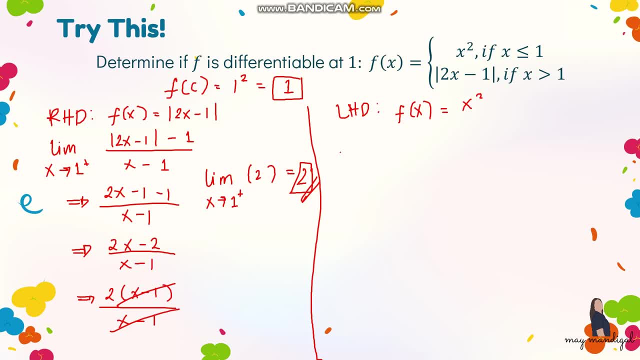 x is less than 1. so let's do the same thing. x approaches 1 from the left this time. so you have f of x minus f of c, which is 1 all over x minus c. and then here you can again simplify: x squared minus 1, that is: 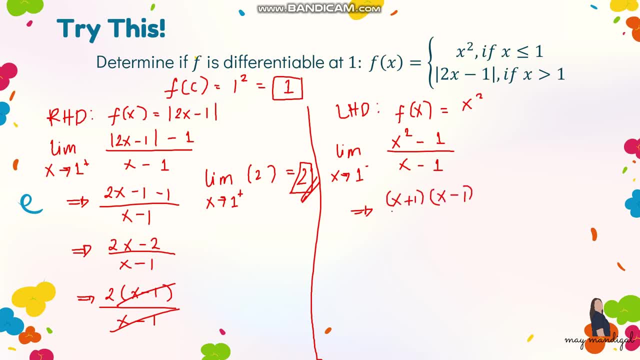 so x plus 1, x minus 1, all over x minus 1. you can cancel this. so you now have x minus 1 or x plus 1. so that's the limit of x as x approaches 1 from the left of x plus 1. so you can just simply. 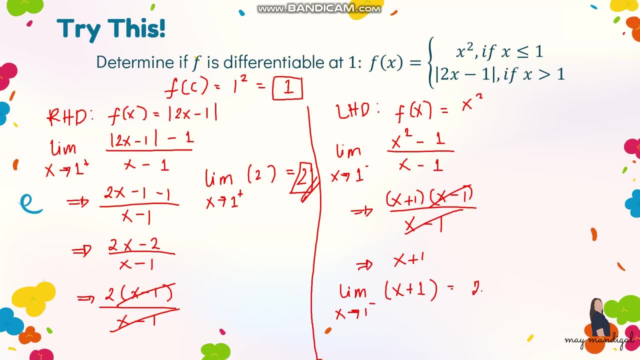 substitute 1 plus 1, so you get 2 as the limit. so, as you can see, the right hand derivative is equal with the left hand derivative. so therefore, our function is differentiable at 1. so therefore, our function is differentiable at 1. so therefore, our function is differentiable. 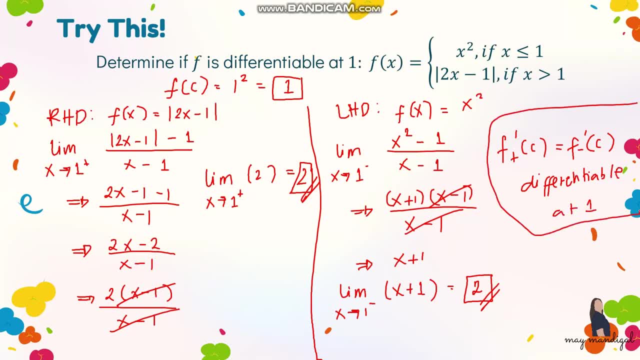 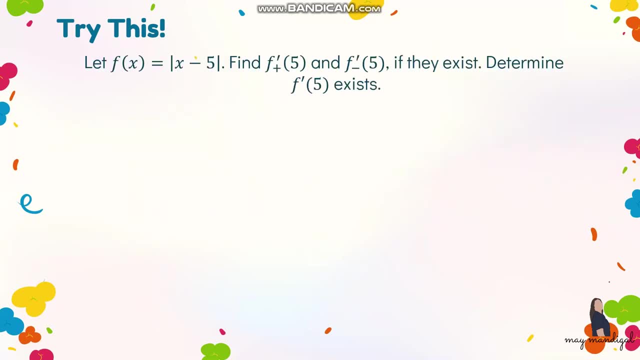 at 1 one, so it is differentiable at one. so if it's differentiable at one, that means our function is also continuous at one. and for our last example, let f of x be equal to absolute value of x minus five. now we have to find the right hand derivative at. x equals five. also the left hand derivative at. 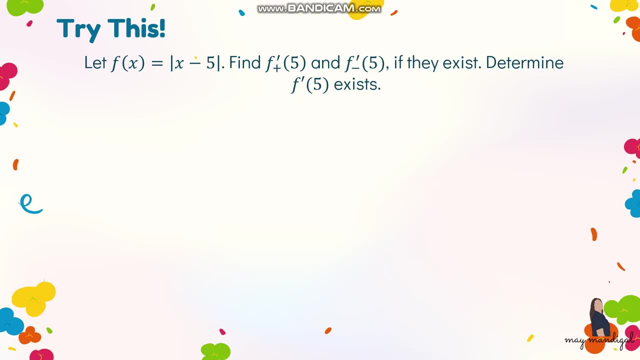 x equals five, and then let's determine if f prime of five exists or if it's differentiable at that particular point. so first, since what we have here, the function that we have, is an absolute value function, let's recall first the things about absolute value function. so let's say we have 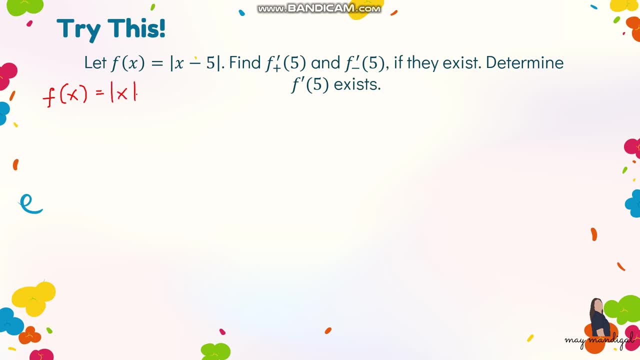 f of x equals absolute value of x. so an absolute value function can be written into a piecewise function because, remember, if it's absolute value, let's say absolute value of x, x can be positive, x can be negative, or the one inside the absolute value symbol can be positive or negative and we still have the 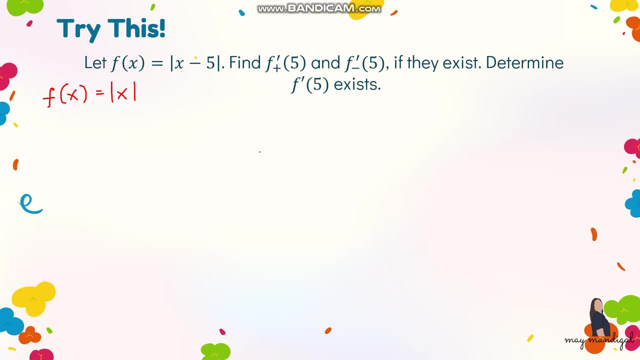 same value if we simplify it. so therefore we can just write it separately, like this again: the one inside our absolute value symbol, which is x, can be positive. that will happen if that function x is greater than or equal to zero, and this one right here will be negative, negative x, if the x that we will put there is, of course, less than zero, or 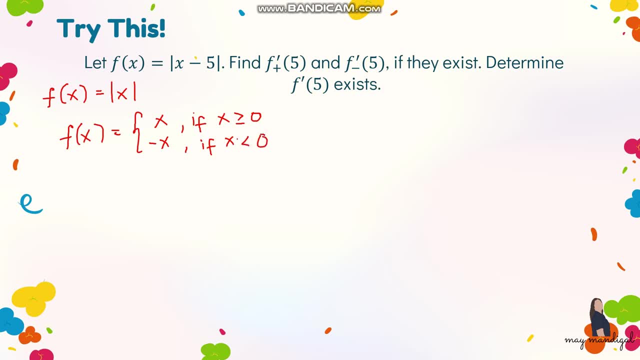 negative value. so this is how we separate or rewrite our absolute value function into a piecewise function. so let's apply the same thing with: f of x equals absolute value of x minus five. so let's write first: absolute value of x minus five. so there, so let's write this as a piecewise. 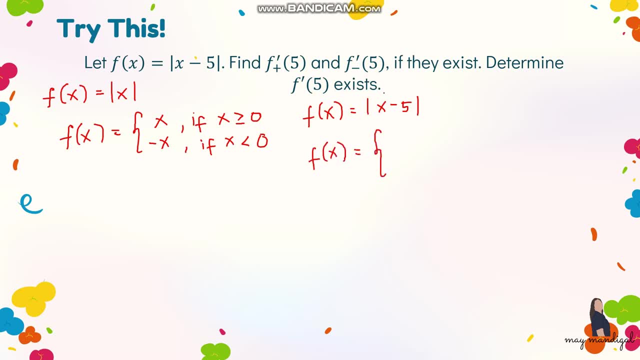 function. so again, this whole term inside x minus five can be positive, given that this term right here, the x minus five, is greater than or equal to zero. so it will only be positive if x minus five itself is greater than or equal to zero, and this whole function will be negative. so negative: x minus five. so it will be. 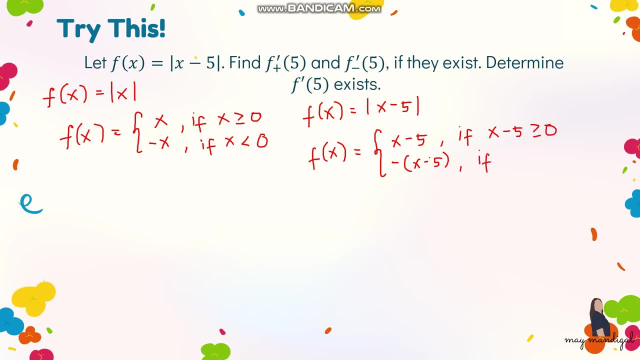 negative if this whole function again is less than zero. okay, so those are the two scenarios that we can write now. next, a thing that you have to do is just to simplify. simplify this piecewise function so we can just write this one x minus five if then it will be positive if we can solve this one. so just move negative. 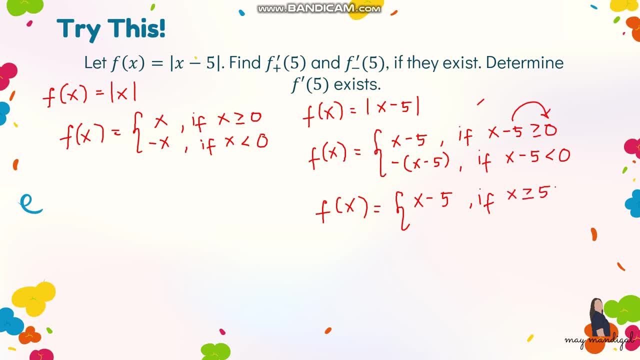 five on the other side. so you have: x is greater than or equal to five. so if it's greater than or equal to five, it will be positive, the output will be positive. this value here inside, and then this one- we can just simplify this one. so we can just simplify this one. so we can just simplify this. 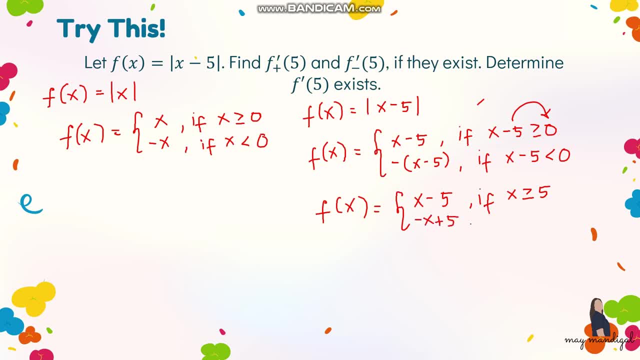 distribute, so negative x plus 5. if then again move negative 5, x is less than 5. okay, so this is now our piecewise function and we will be using this to check if the right hand and the left hand derivative exist. so let's try to solve for the right hand derivative. okay, but first what is f of? 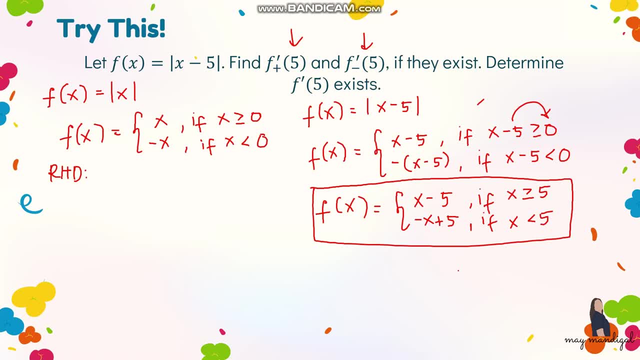 c. so our c is 5. so we will be using this one, the first sub function, to solve for f of c. so f of 5 is equal to 5 minus 5, which is equal to 0. so, remember, our f of c is equal to 5. so now, 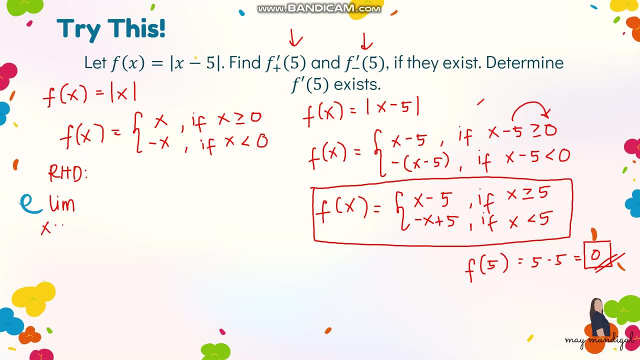 let's substitute. so we have limit as x approaches c, which is 5 from the right f of x, since what we want is from the right or the right hand derivative. so we will be using the first sub function. so that is x minus 5, minus f of c, which is 0 all over x minus c. 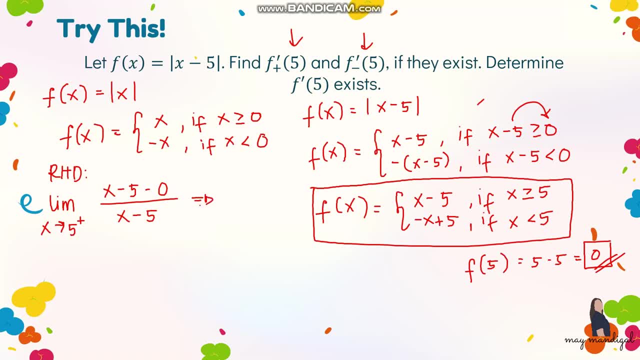 so if you simplify this, so we now have x minus 5 over x minus 5, or this will be cancelled. therefore, what we will have now is limit of 1 as x approaches 5 from the right, and we know, since this is constant, the limit is one. okay, so that is now our right hand derivative. now let's solve for. 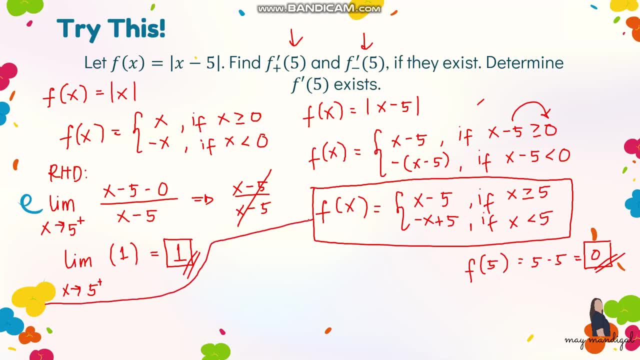 the left hand derivative. so let's just write here: left hand derivative. so for the left hand derivative. so we have limit: as x approaches five from the left, our f of x to use, or the sub function to use, will be the second one. so we have negative x plus five minus zero, which is f of 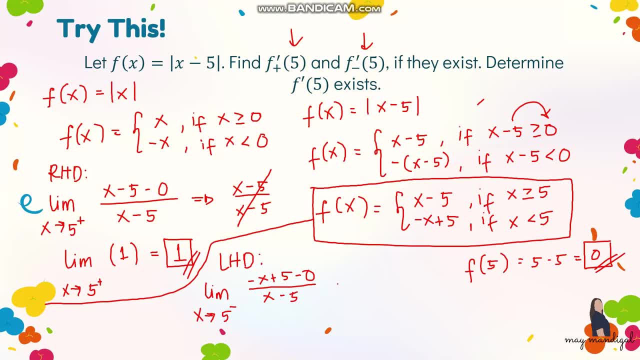 c all over x minus five, and then from here this one, it's negative, x plus five over x minus five. now, from here we can simplify this by factoring out the negative one, so we have x minus five all over x minus five, something like that. so this can be cancelled out. therefore, we now have limit of negative one as x approaches five.